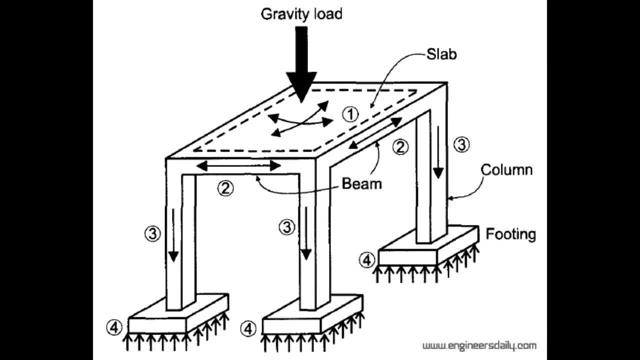 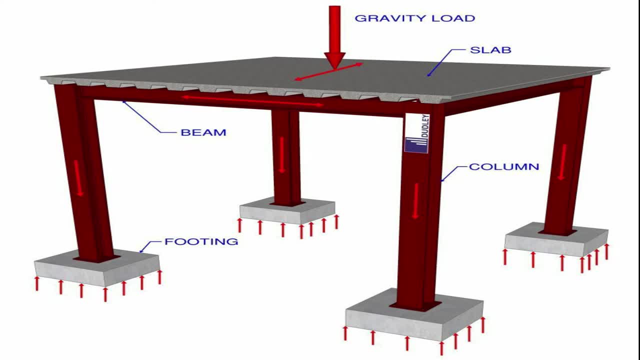 This figure shows an isometric view of a concrete structure and a gravity load path path. The vertical gravity load acts on a slab which transfers the load to the beams, which in turn transfer the load to the columns and then down to the foundations. The gravity load path. 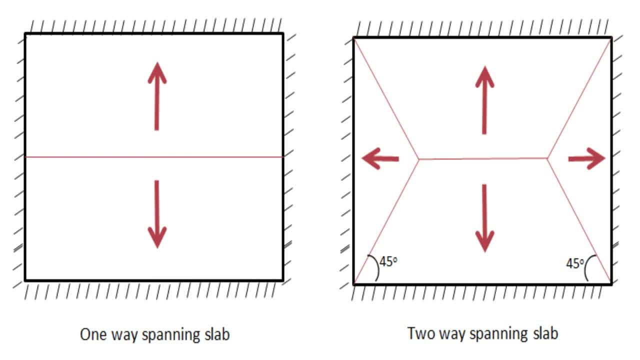 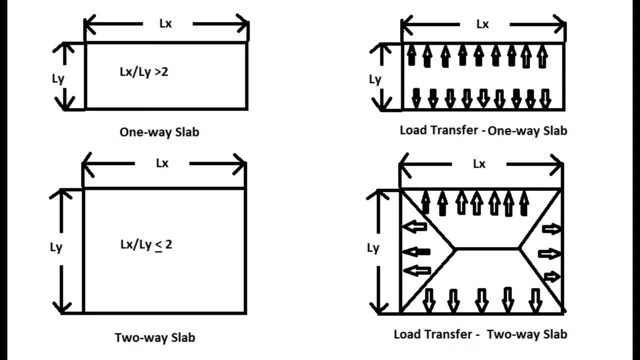 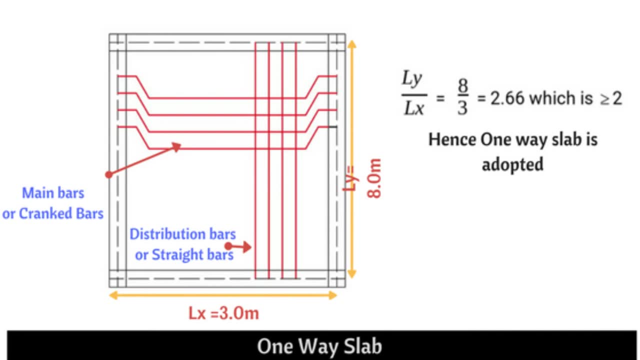 depends on the type of floor slab, that is, whether a slab is a one-way or a two-way system. In the one-way system, the effect of external loads is transferred primarily in one direction. The slab beam and girder floor is an example of a one-way system: The gravity load 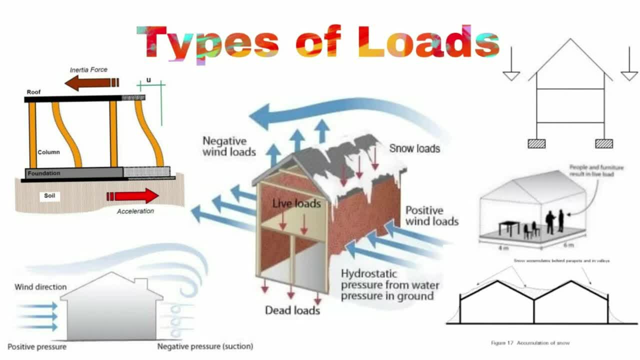 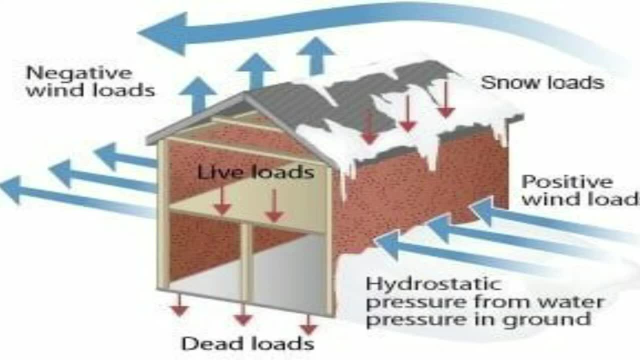 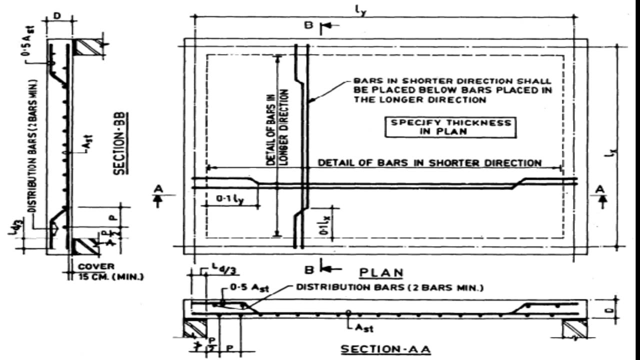 acting on this system is transferred from the slab to the beams and then to the girders. Finally, the girders transfer the load to the columns. The load path in a two-way system is not as clearly defined. The slab transfers gravity load in two perpendicular directions. however, 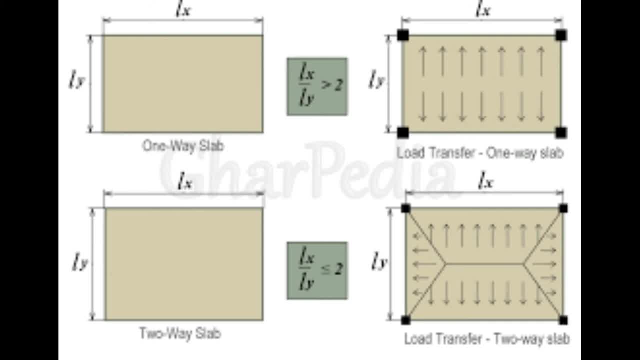 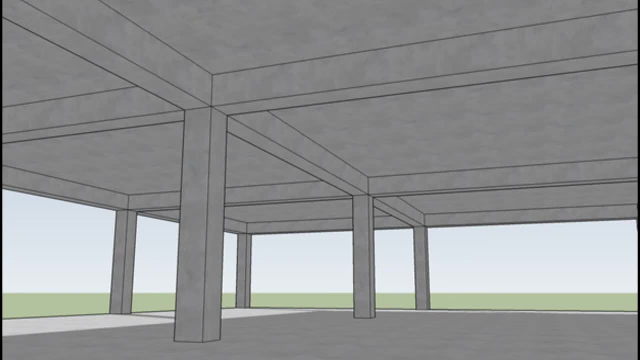 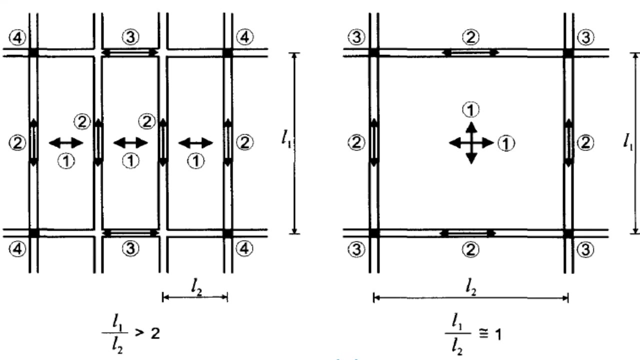 the omegle carried in each direction depends on the ratio of span lengths in the two directions, the type of end supports and other factors. for example, in the slab with beam system shown in figure, the load is transferred from the slab to the beams aligned in the two directions and then to the columns. that's all about the 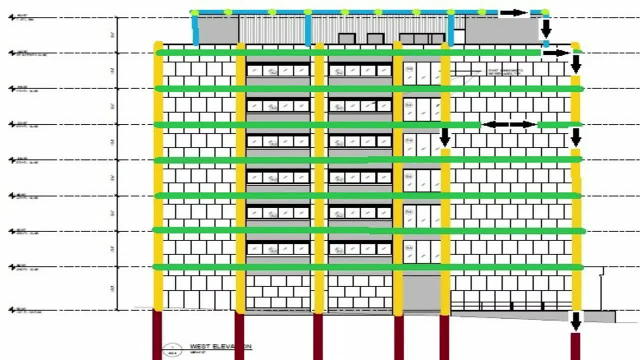 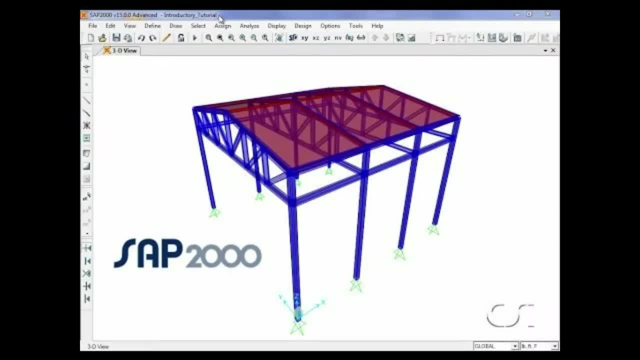 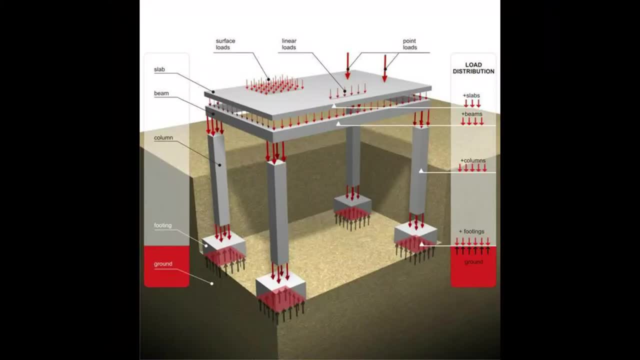 gravity load path and then the type 2 lateral load path. the lateral load path is the way lateral loads, which are mainly due to wind and earthquakes, are transferred through a building. the primary elements of a lateral load path are as follows: vertical components which are in the path are shear walls and. 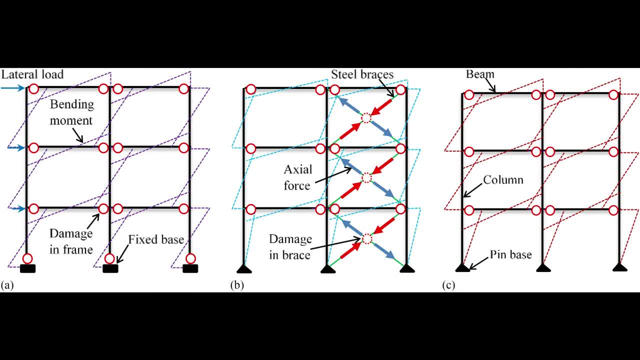 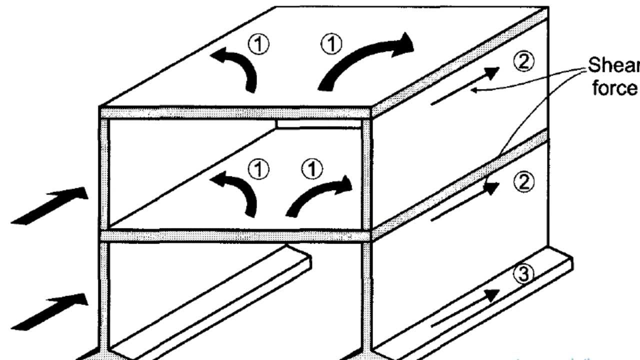 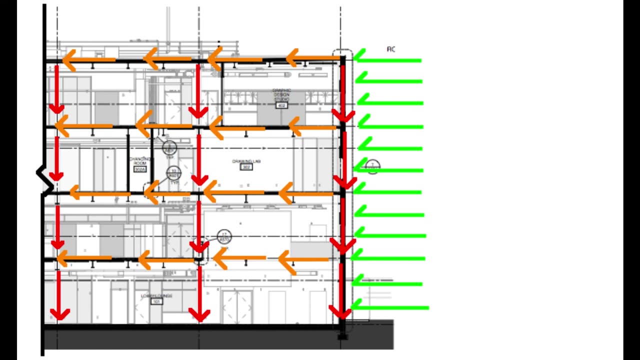 frames and then the horizontal components in the path: our roof, floors and foundations. the figure on the screen shows a reinforced concrete structure and the hom ні 내용 constituting the lateral load path. the roof and floor systems transfer the load to the walls, which in turn transfer the load to the foundations in the final